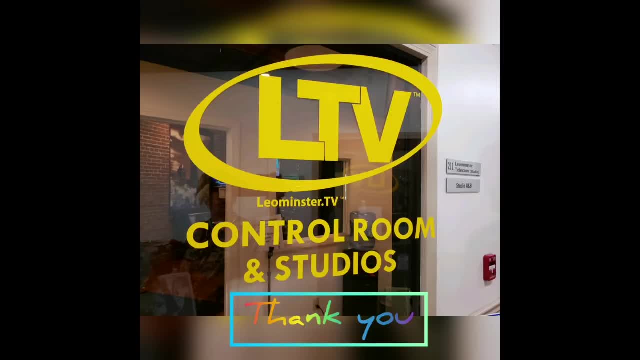 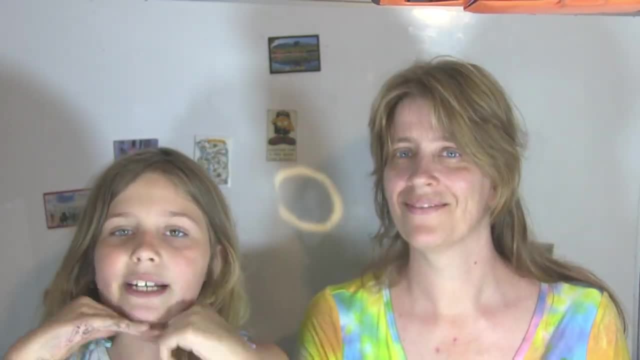 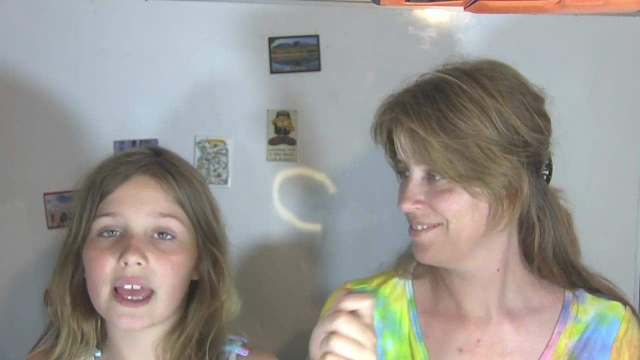 Hello and welcome to Dreaming English, where we are teaching English in a natural way. My name is Katerina and this is my mom, Rochelle, and we want to thank LATV Women's Directs for this channel for lending us equipment and Pablo Dreaming Spanish for helping us. 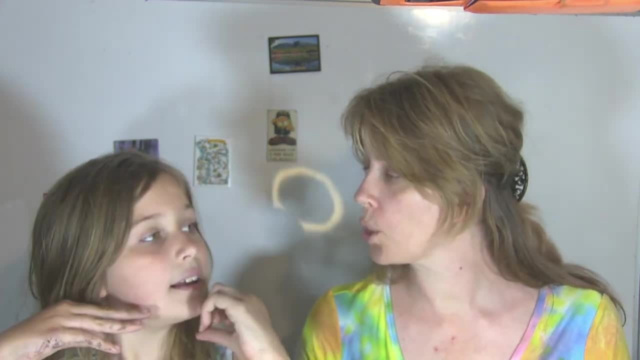 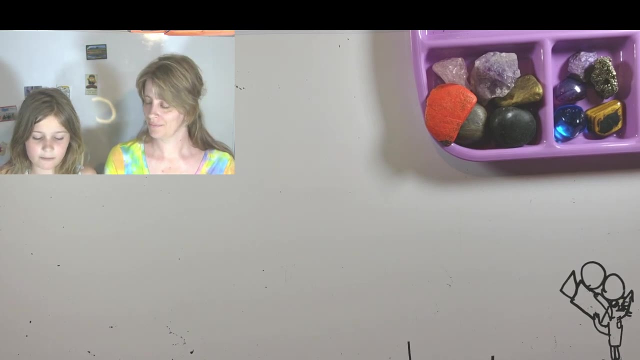 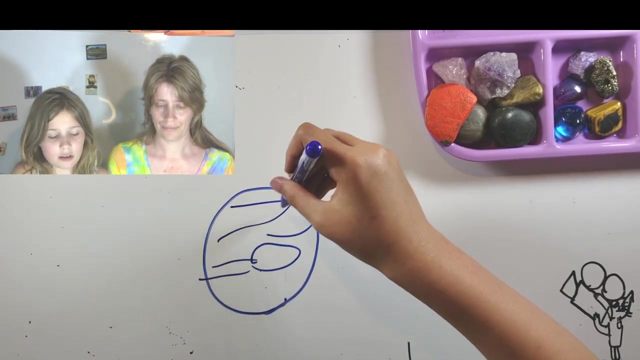 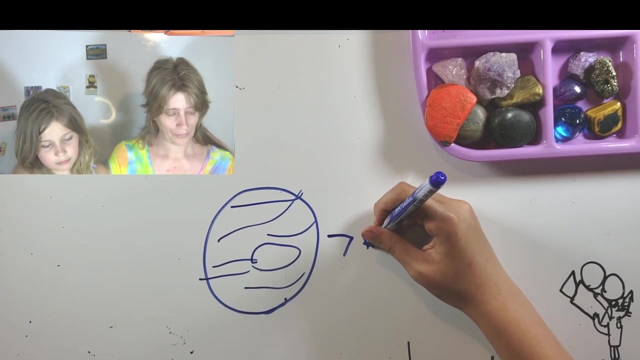 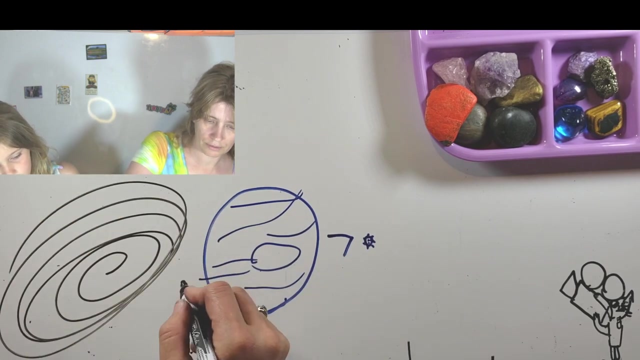 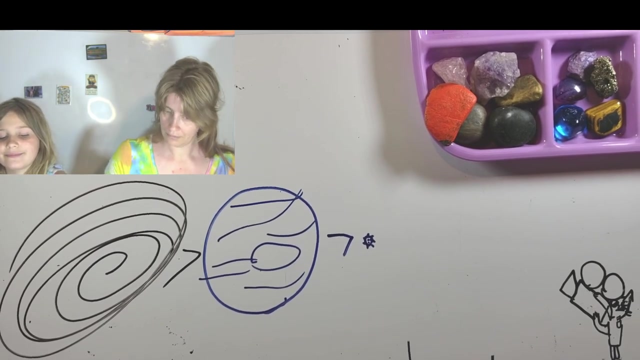 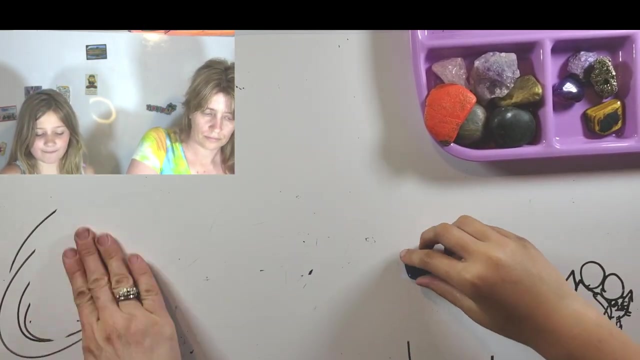 inspire this channel. Today we're going to be doing colors and sizes, like big and small. Like this is a planet, it's very big compared to a little tiny microbe, And then a galaxy. So for the colors, this is a rock. it is blue. 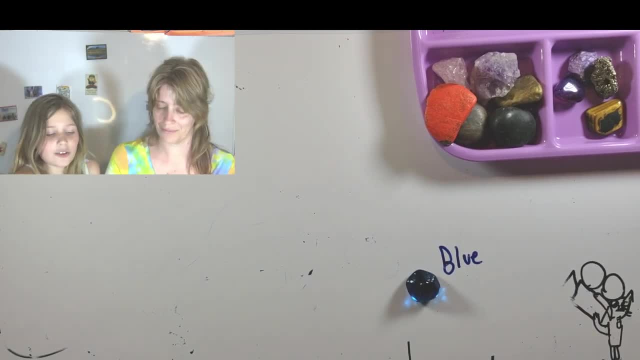 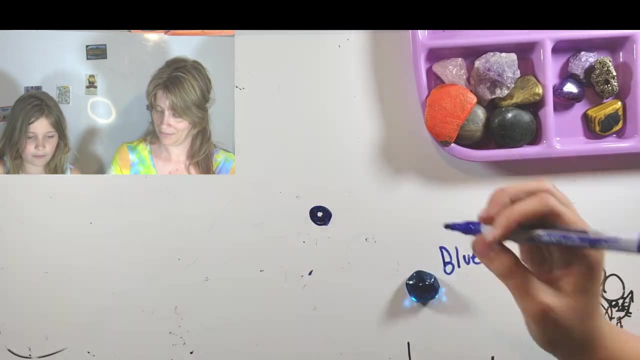 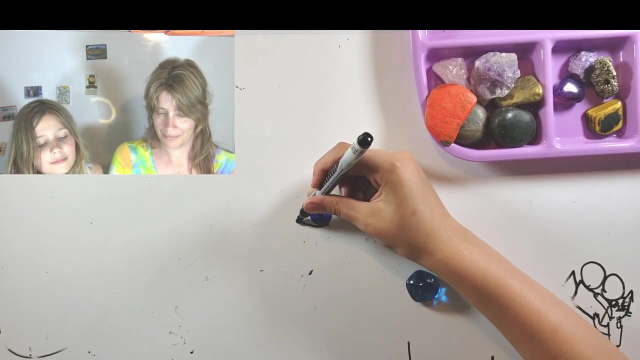 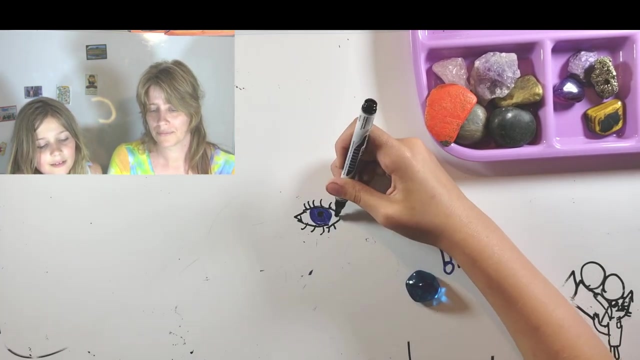 Like my mom's eyes, they are blue. Her eyes are blue, As you can see. I am writing in blue My eyes. I can see with my blue eyes. Yeah, this is my mom's eye. This is from my mom. 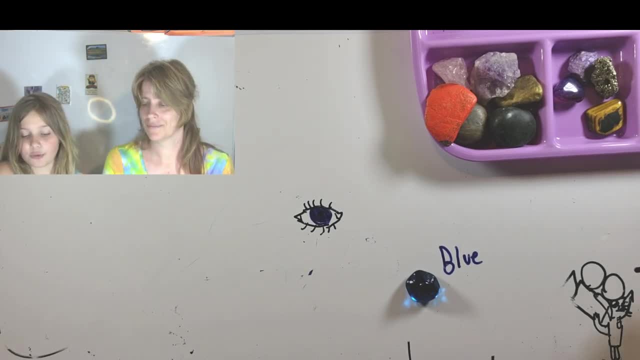 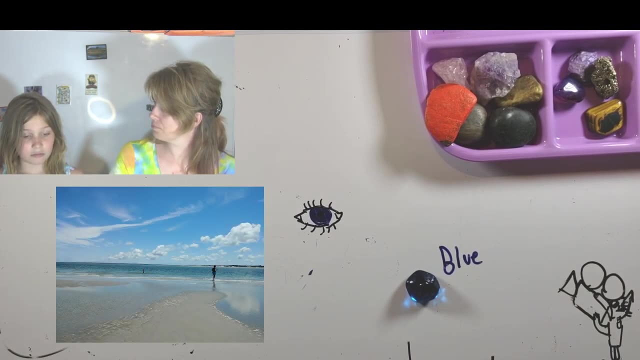 So there are other blue things. So what are other blue things? What other blue things are there in the world? There's The ocean. Yeah, the ocean is blue, with fish. The sky, the sky above us, is blue. 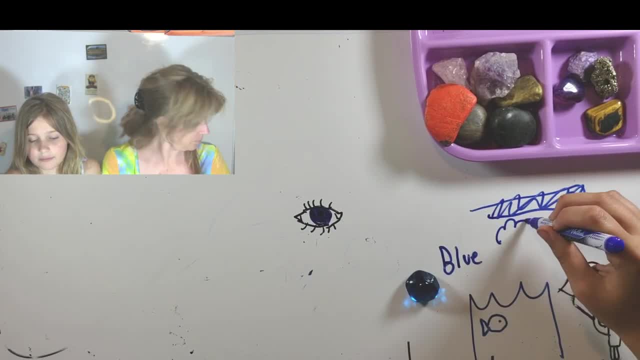 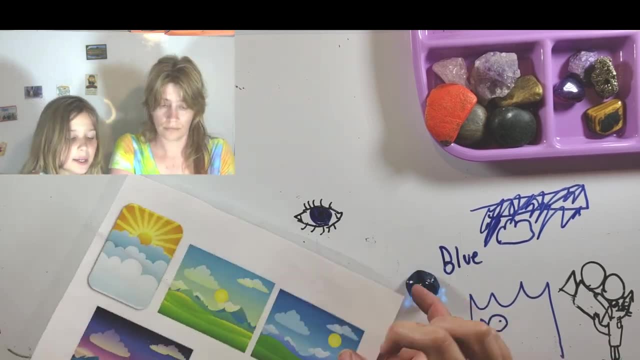 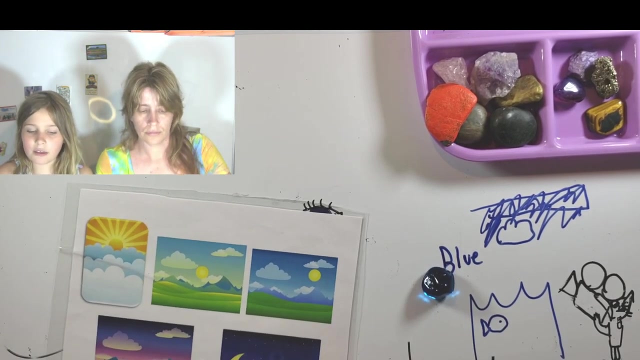 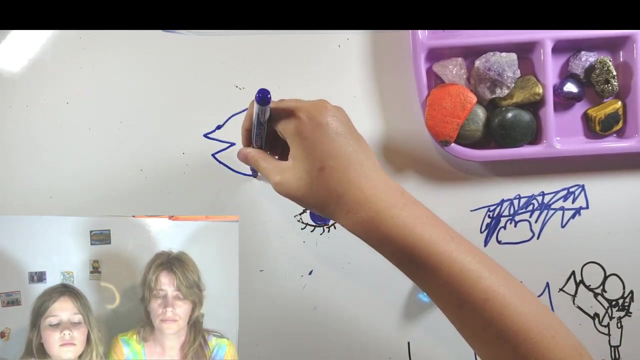 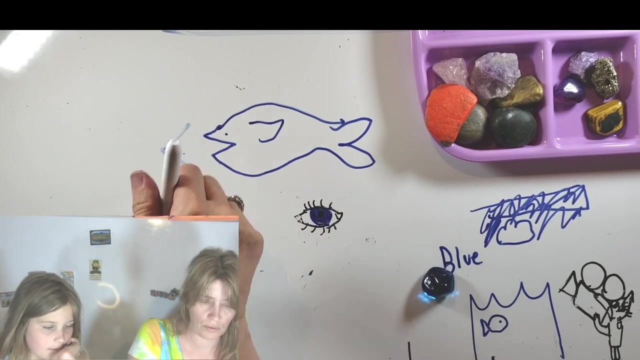 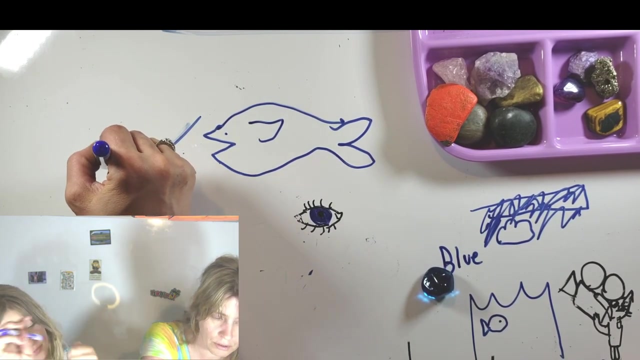 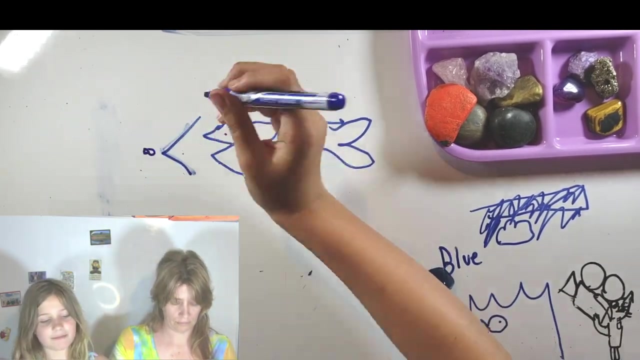 Yeah, the sky with the clouds- Let's see. See, The sky is above- is blue. Want to know what else is blue? A big blue whale, And a blue whale is bigger than a small fish. A fish is much smaller than that compared to a blue whale. it's like this: 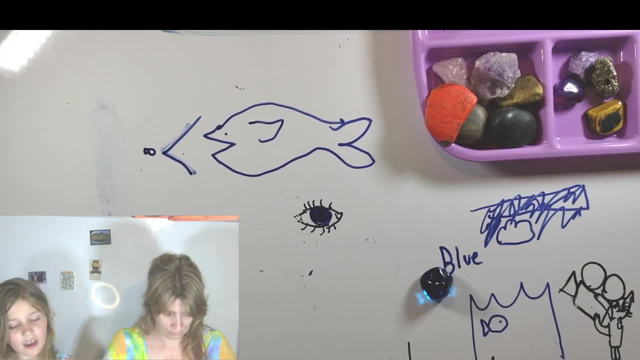 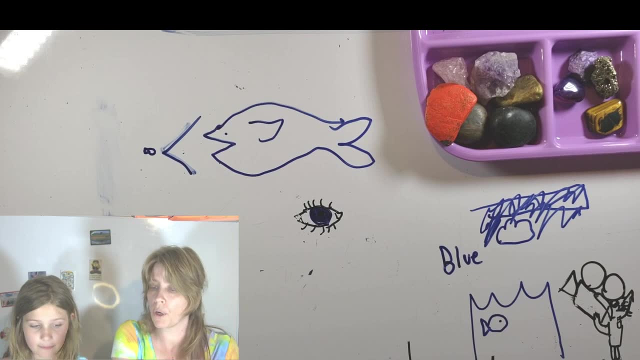 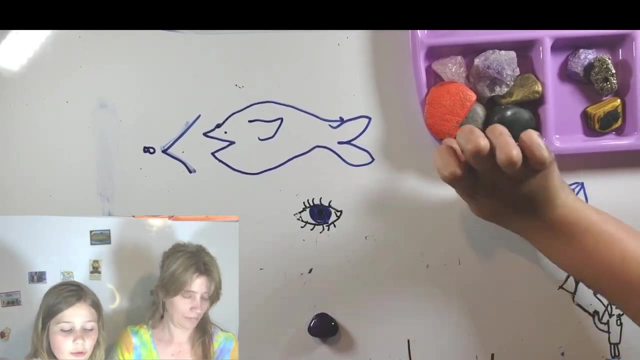 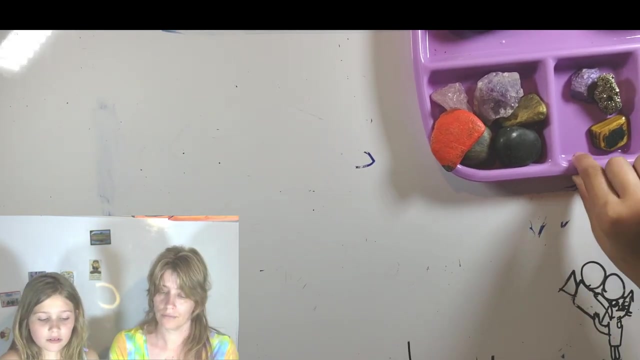 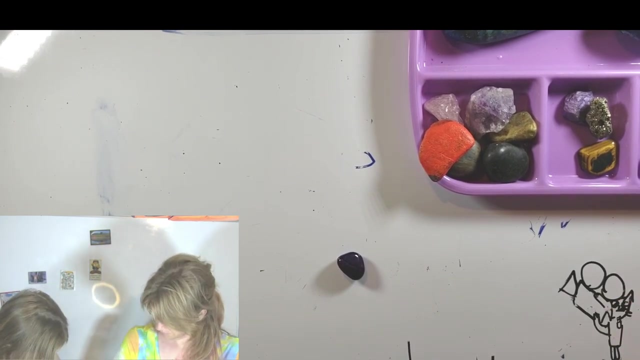 Maybe even smaller than that, probably. So now let us look at another color. We'll have to use purple, but we don't have a purple marker. So there are many things that are purple. For instance, The tray here is purple and something else is purple. I have some purple on my shirt. 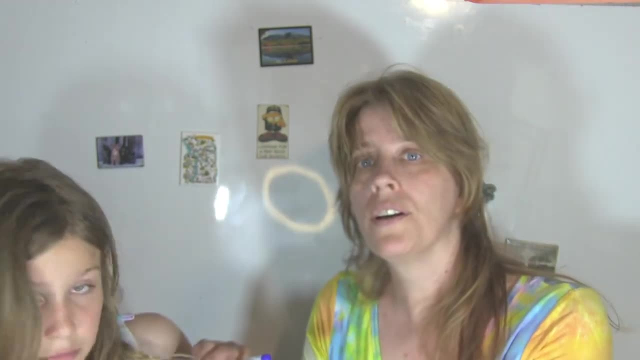 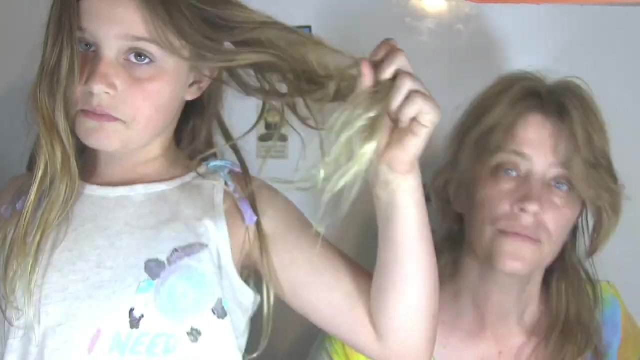 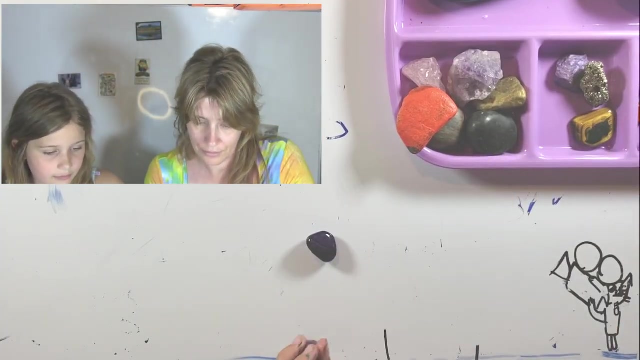 here. Let me make sure that we can see it. your shirt is very much lower, so stand up and show the purple. I have a little bit of purple around here on my shirt and there are several purple rocks here. Okay, Okay. 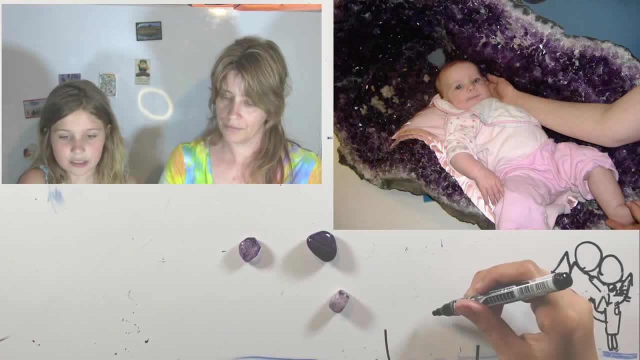 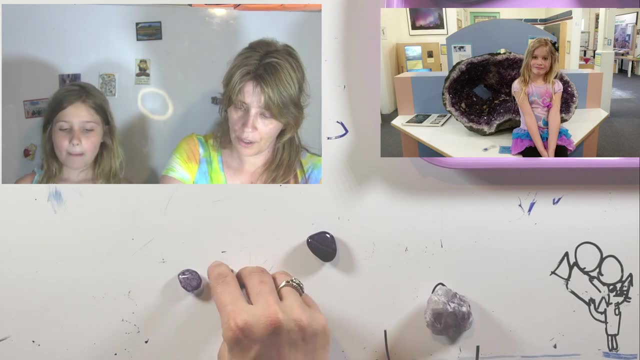 This one is amethyst, Amethyst is purple And, Let's see, This one Is also amethyst. These are both the same type of rocks, Now, And this one is bigger. right Yeah, This rock is bigger than this rock. 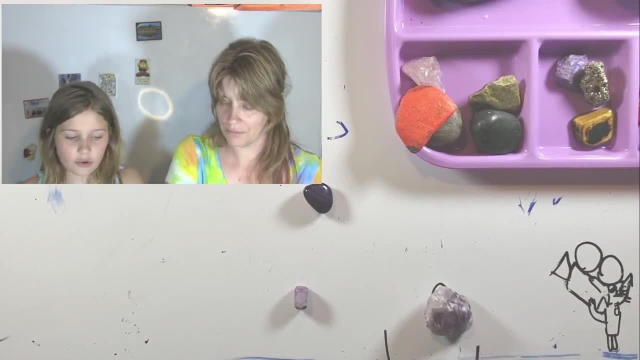 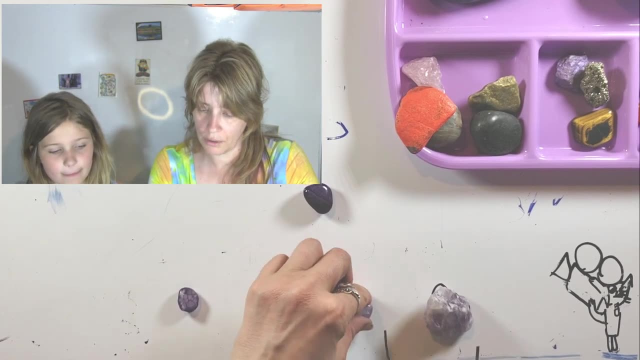 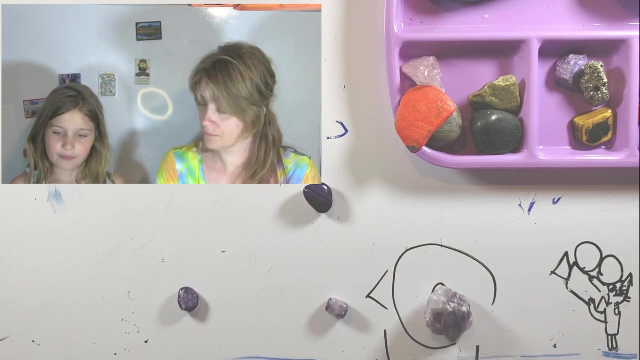 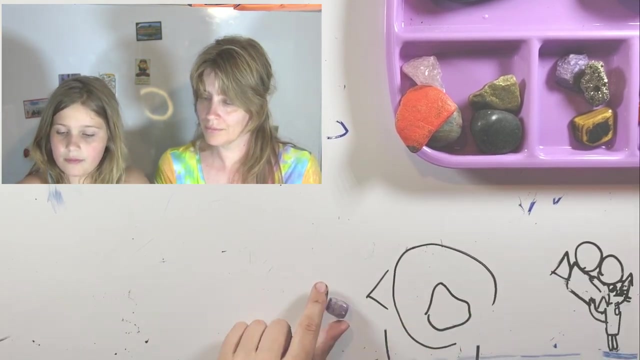 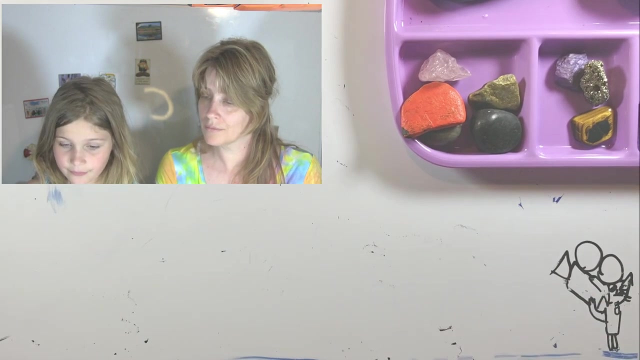 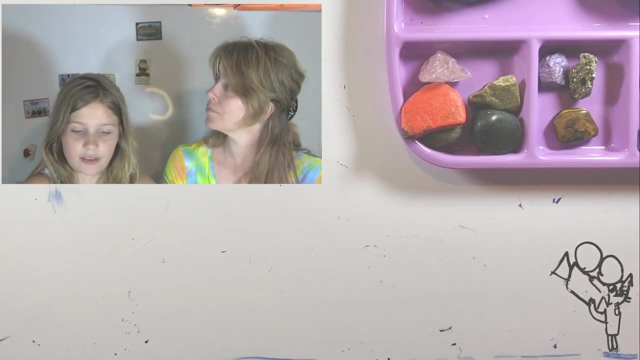 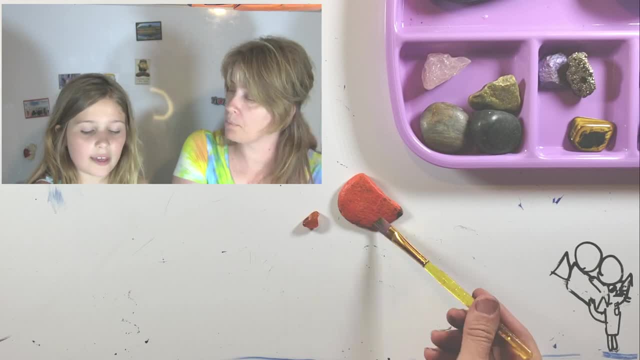 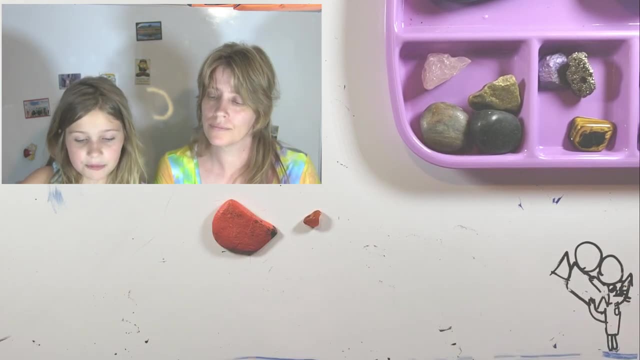 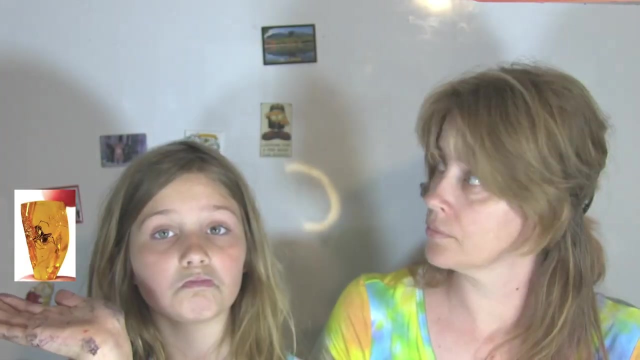 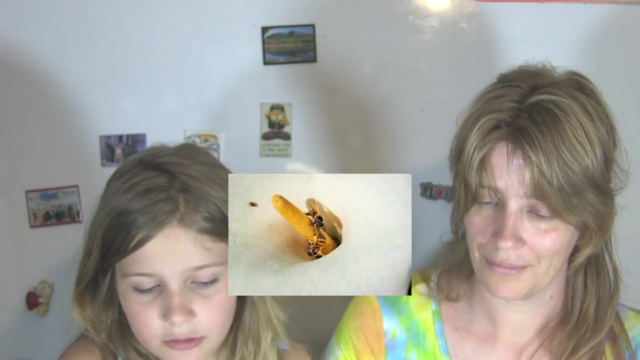 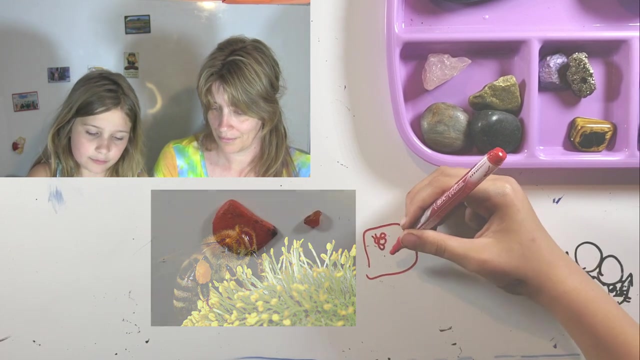 Orange paint. It's a mixture of two different colors. Yeah Yeah, somebody took orange paint and painted the rock Something else. that is orange. another orange rock is amber. Here's some amber. here's another example of amber with bees stuck in it. 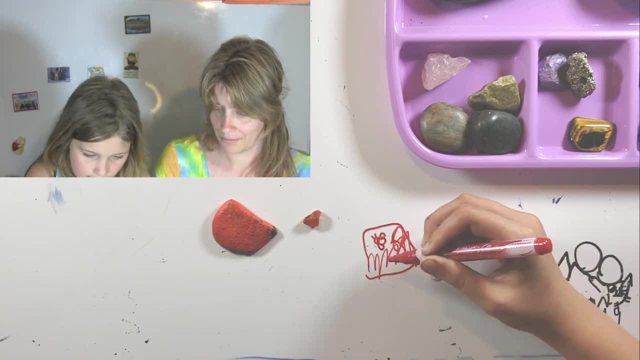 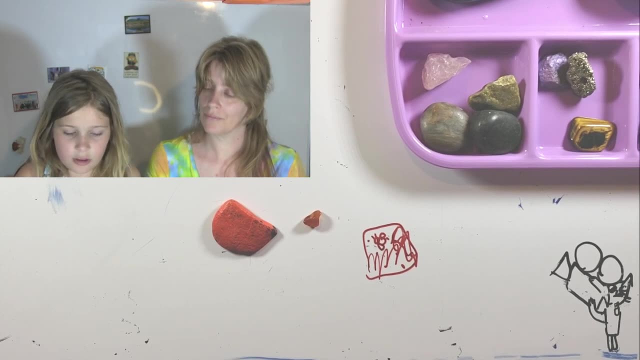 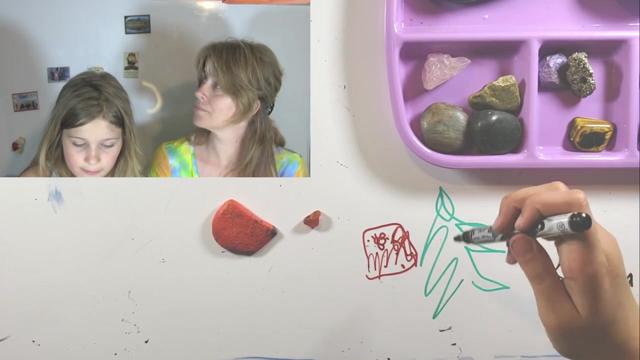 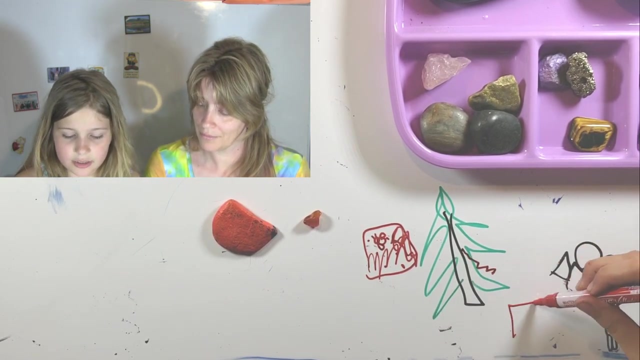 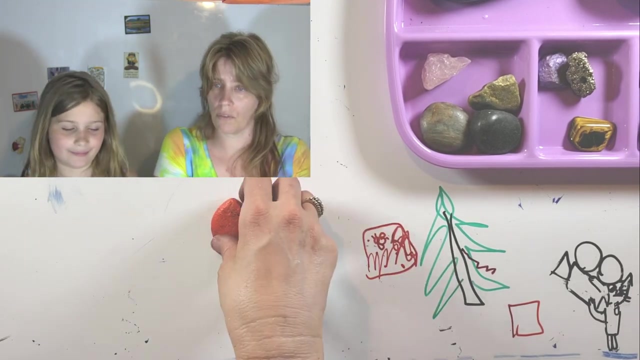 And other little things. Amber is when sap comes out of a tree, a tree, when sap comes out and hardens for many, many years, It's very hard. It's hard, Yeah, Like a doodle, Like a rock. 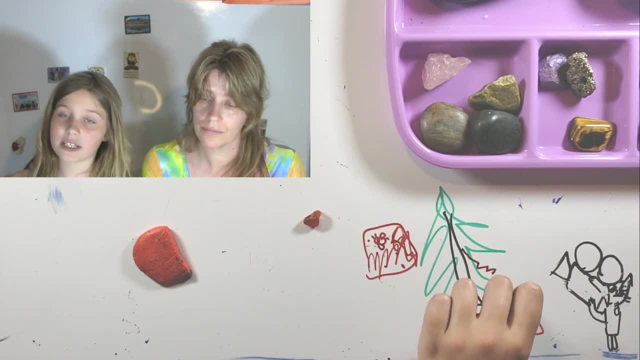 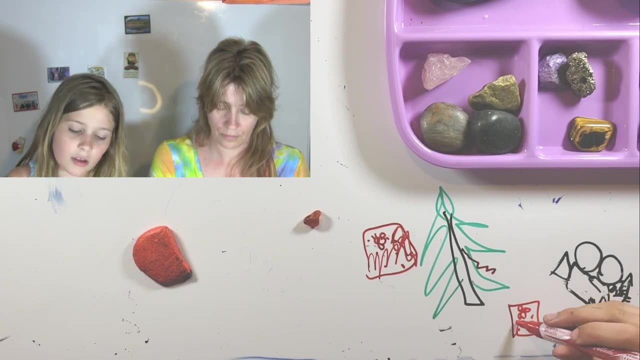 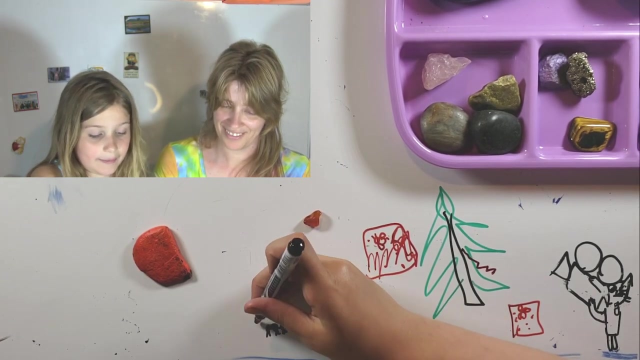 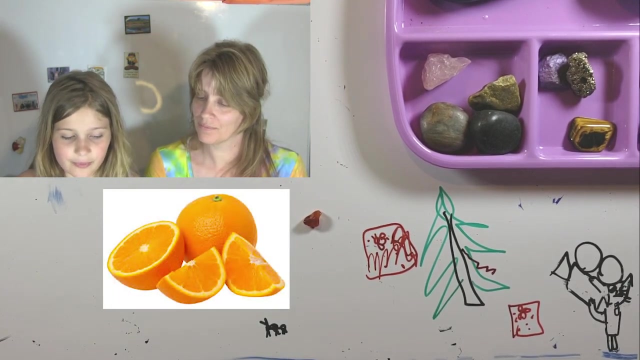 It's very hard, so it becomes a type of rock known as amber, and then bugs can get stuck in the amber And these little ants Too many legs. Wait, I forgot that. Alright, so Now that is the color orange. 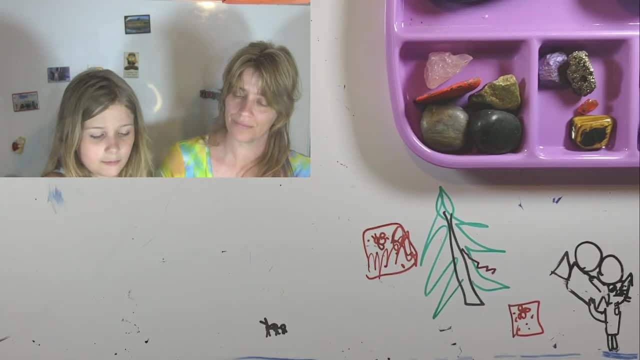 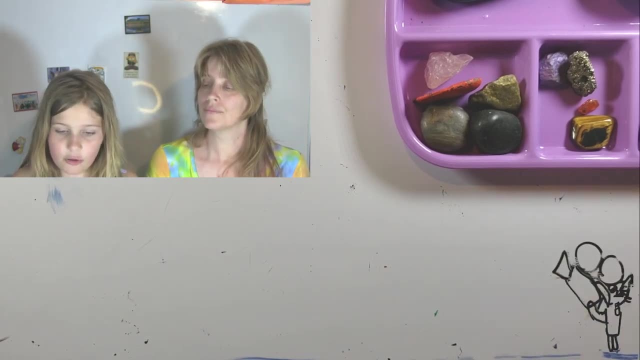 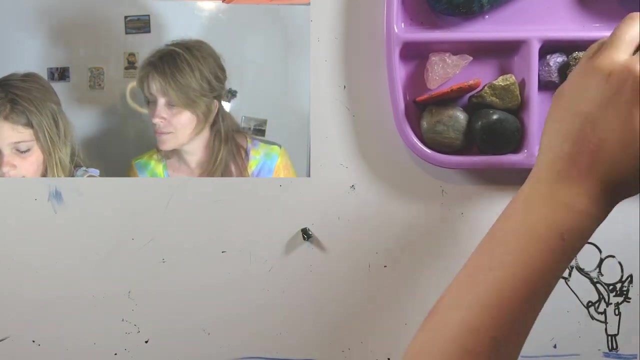 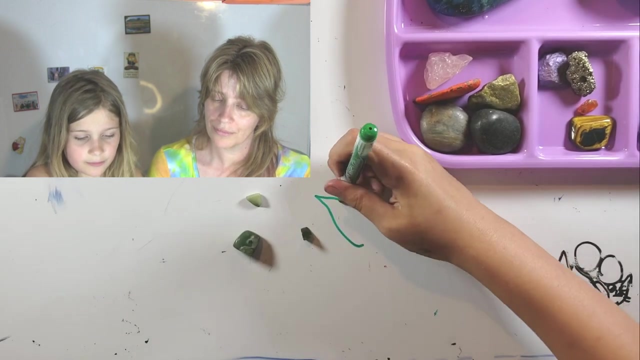 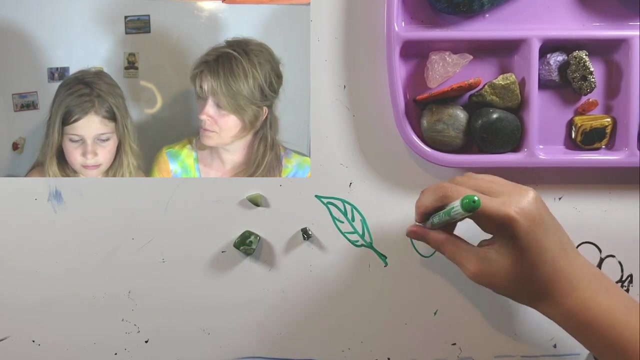 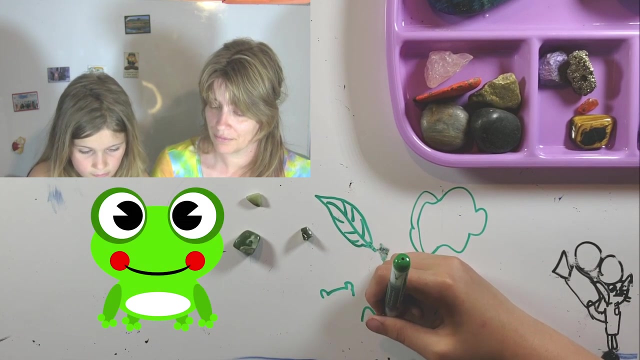 So there are other colors too. So this color is green. So there are some green things like the leaves on trees, Okay, Okay, Okay, Okay, Okay Okay. And frogs, Yes, Sometimes. Sometimes, I mean usually. 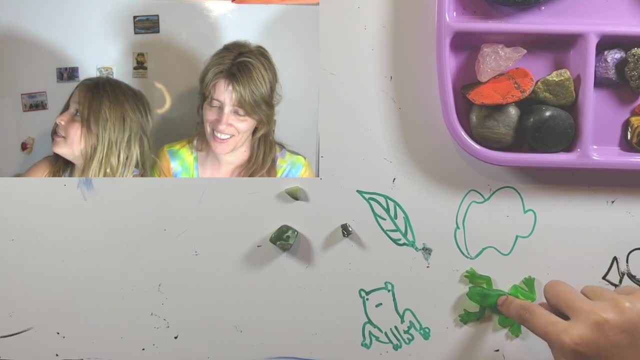 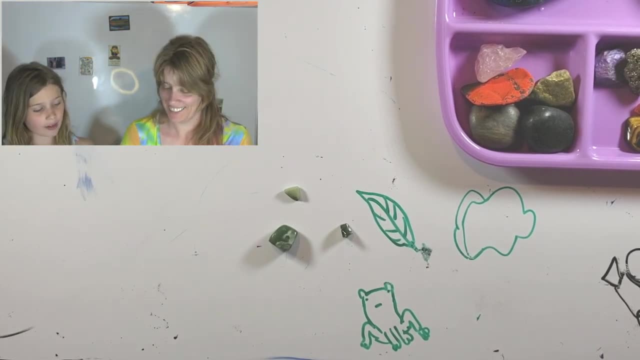 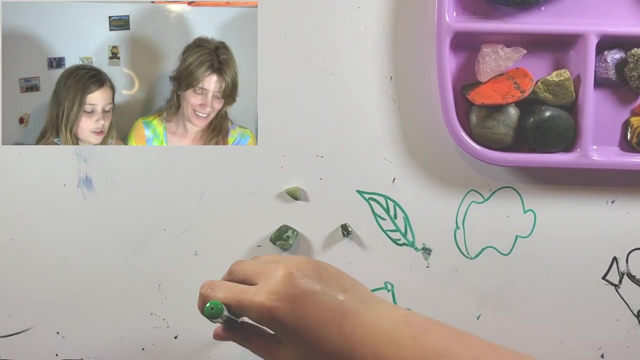 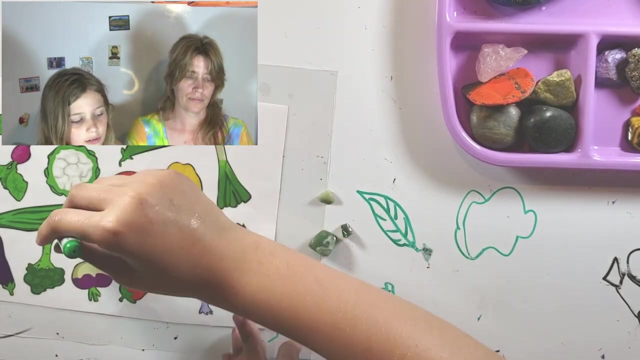 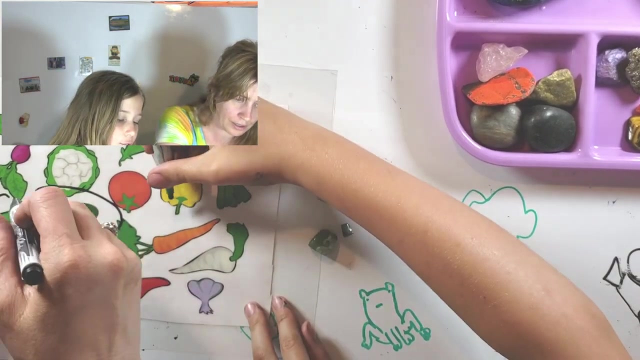 Frogs are green. Oh yes, Here we go, we have a frog: Ribbit, ribbit, ribbit. When you go to the store, there are some vegetables that are green. Many vegetables are green and most of them have green stems. That is the color green.